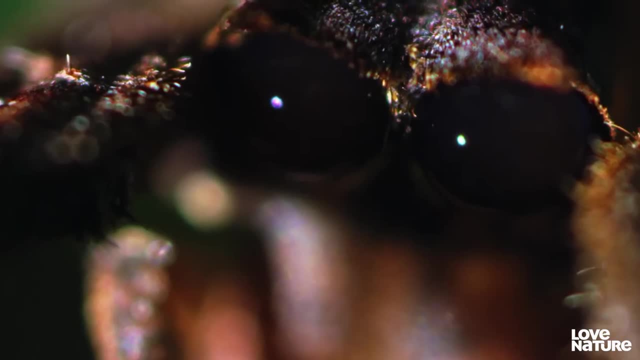 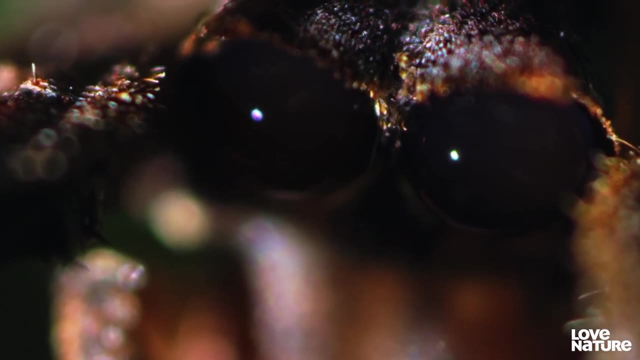 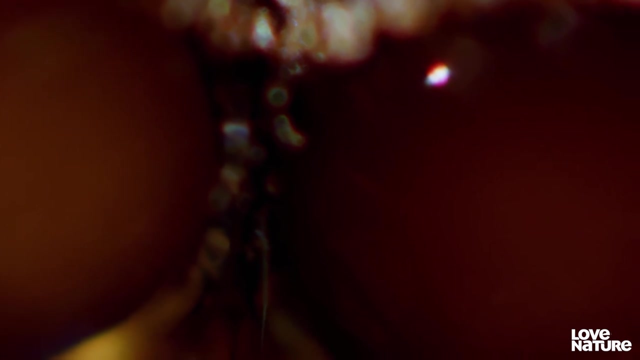 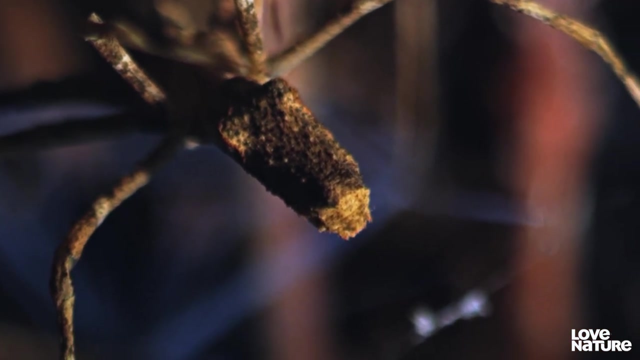 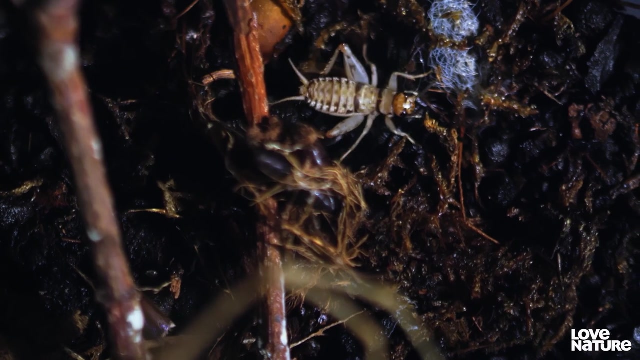 Like all arachnids, it has eight eyes. The huge front-facing ones act like night-vision goggles, allowing it to see in the dark better than cats or owls. To help it line up the perfect shot, it deposits blobs of white faeces as markers on the forest floor below. 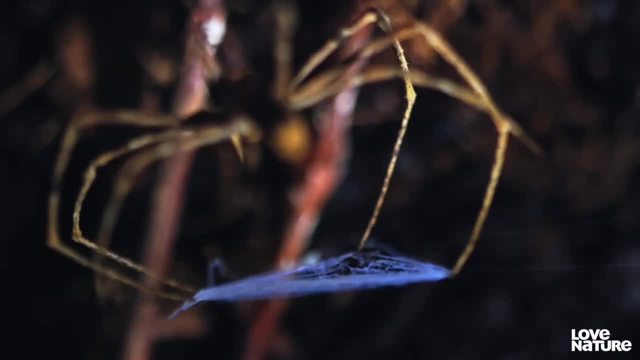 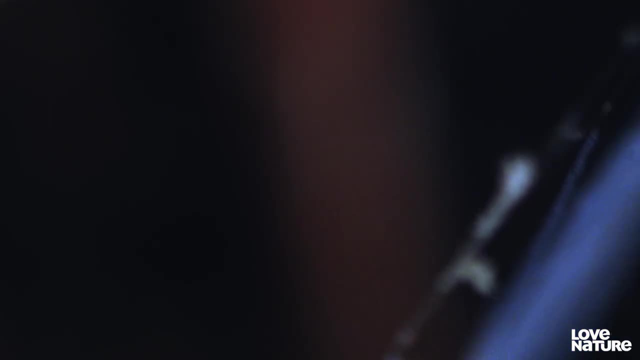 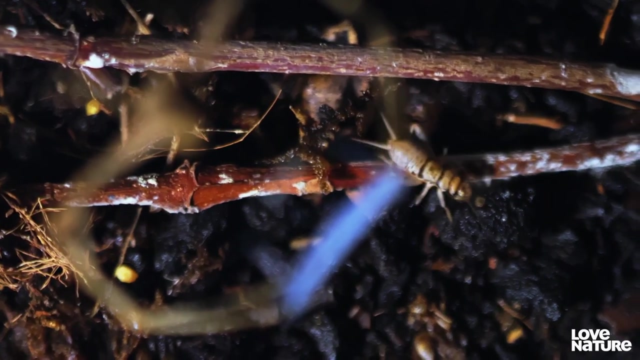 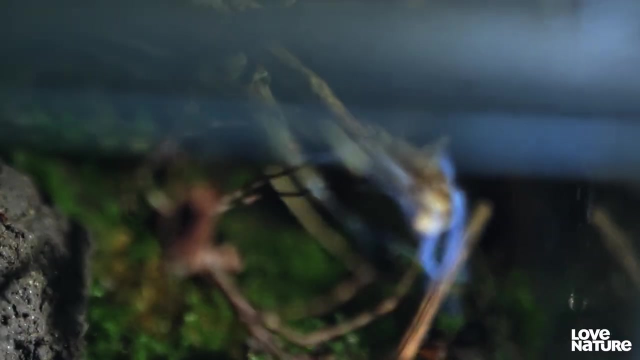 If the unlucky bug should look up, this is the last thing it would see. The spider stretches its net to as much as four times its original size And pounces With its victim entangled. it can deliver its lethal venom at leisure. 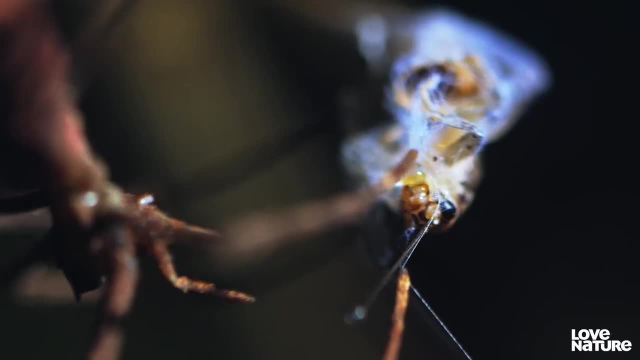 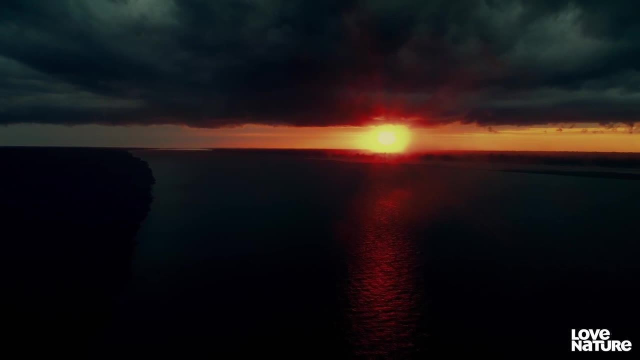 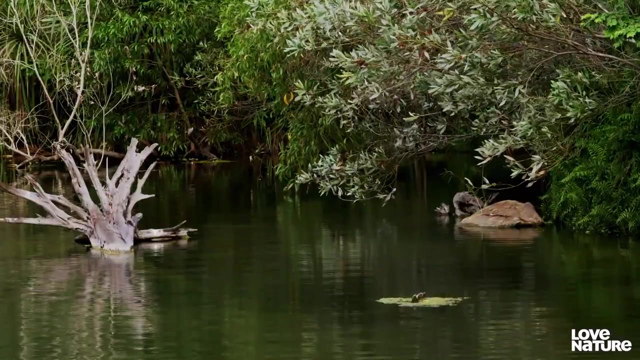 It's a remarkable display of weaponry And uses far less energy than building a large static net. A handful of creatures take hunting ingenuity even further, displaying highly evolved ways of taking down prey. The mangrove, swamps and rivers of North Australia are home to an unusual fish. 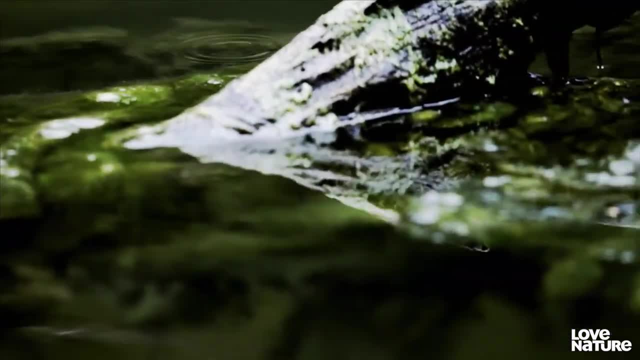 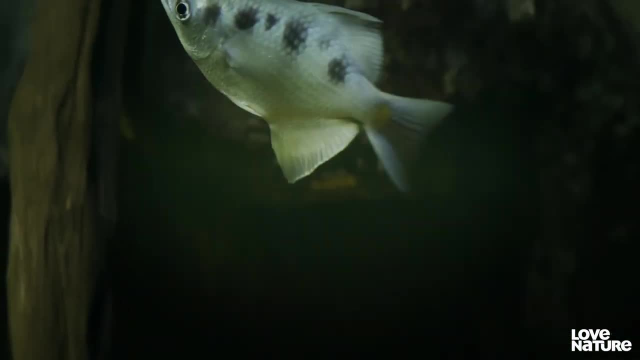 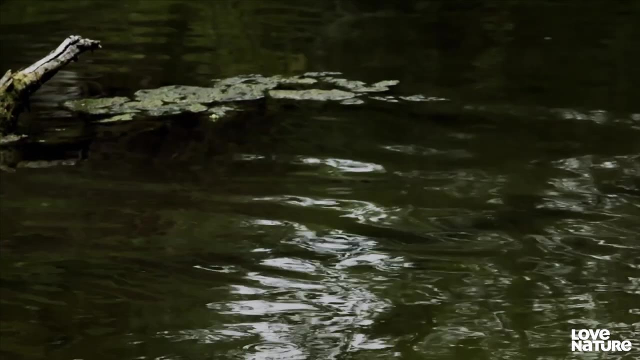 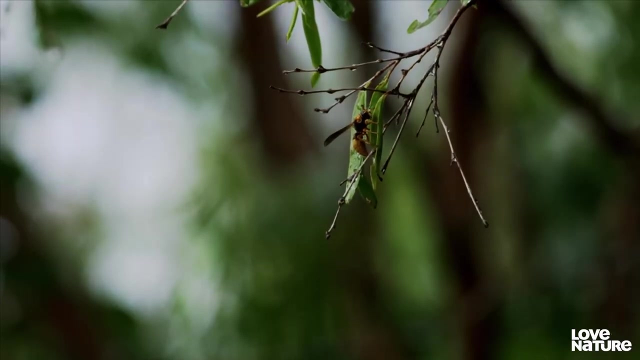 Camouflaged to blend in with the dappled shade cast by the dense foliage. it's on the hunt for its favourite meal: Insects. The fact that there are no bugs in reach doesn't faze this fish, because it's armed and dangerous. 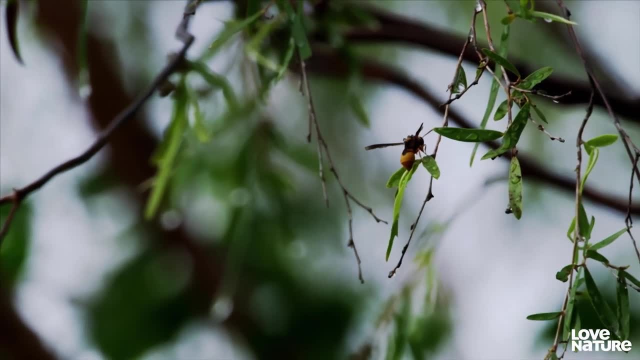 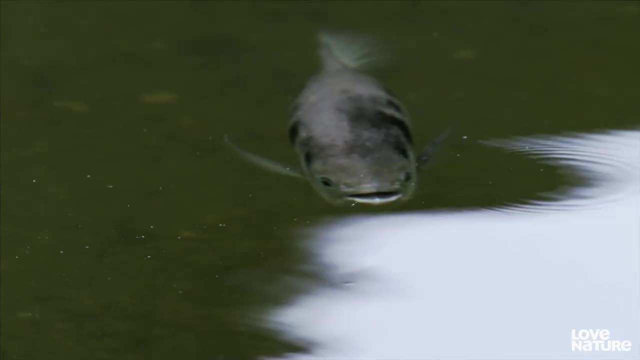 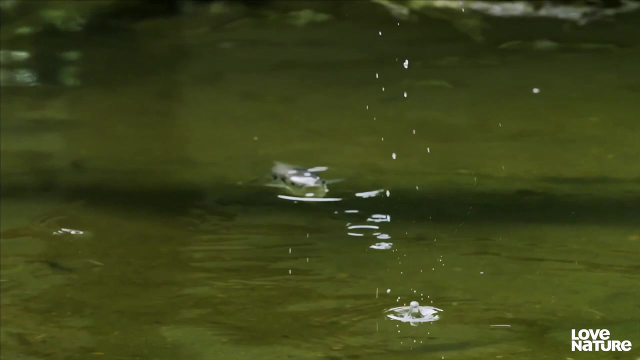 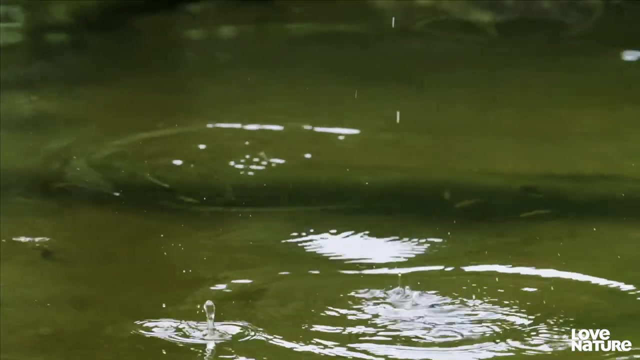 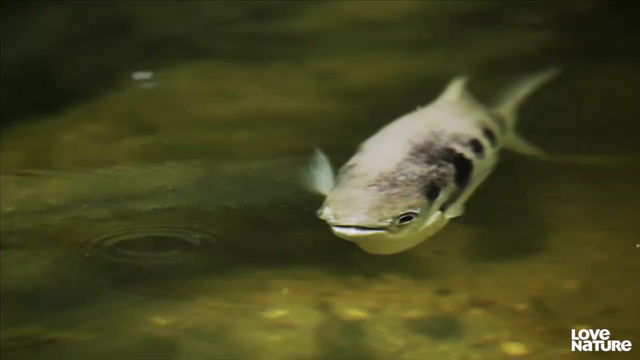 It's also known for its. It has sniper-like accuracy, Hitting targets up to six and a half feet away. How a fish just four inches long can do this was a mystery. But the fish's strength is share. this was a mystery until recently. 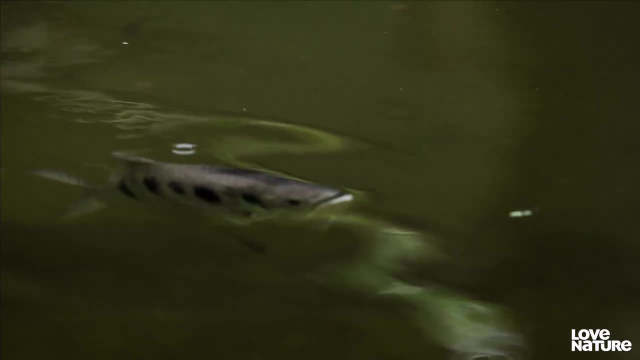 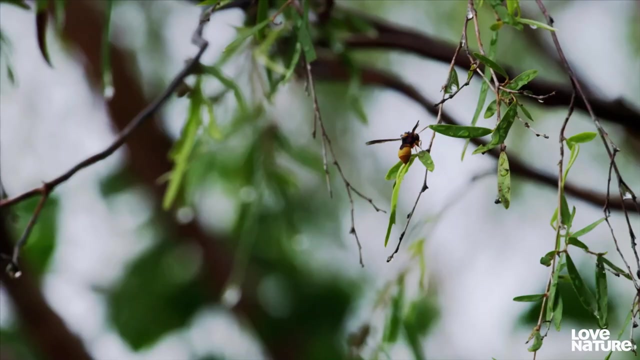 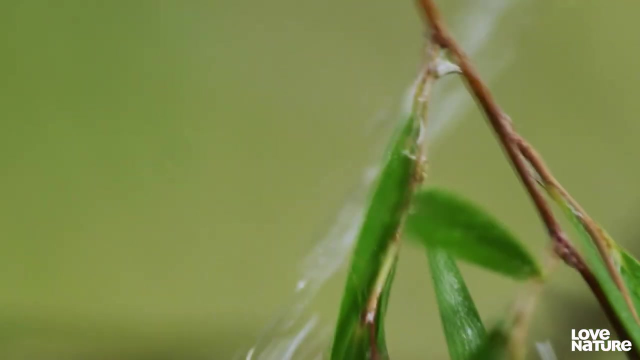 Scientific studies revealed the archerfish can change the velocity and power of the water it spits out. By changing the shape of its mouth, it turbo charges the back end of the water stream. This high velocity water then catches up with the front of the water stream. 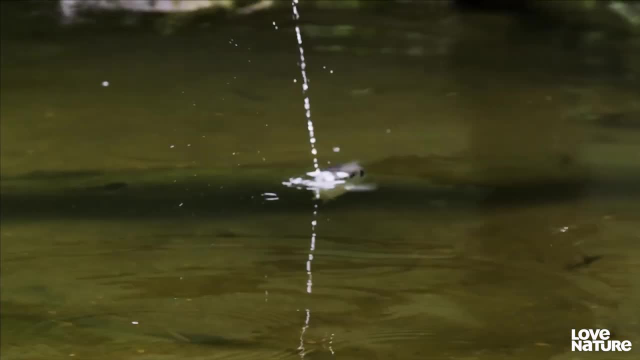 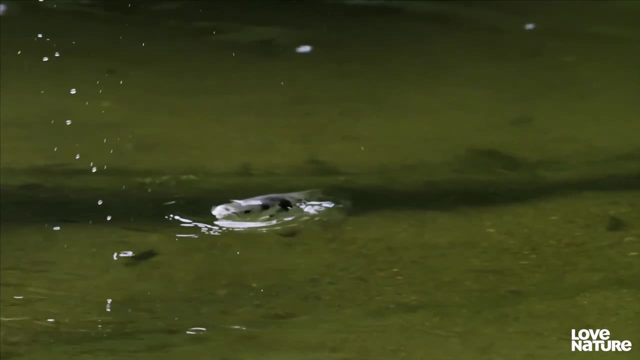 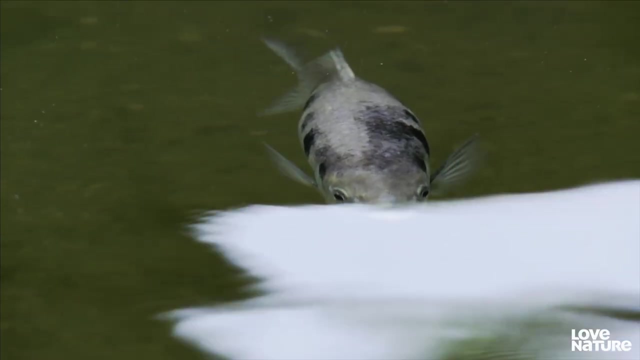 and the whole lot hits the victim with maximum force. Its near perfect hit rate is just as startling. This hotshot can adjust its aim to account for the distortion of the water and assess the effects of gravity on the trajectory of its missile. It can even estimate the weight of its target. 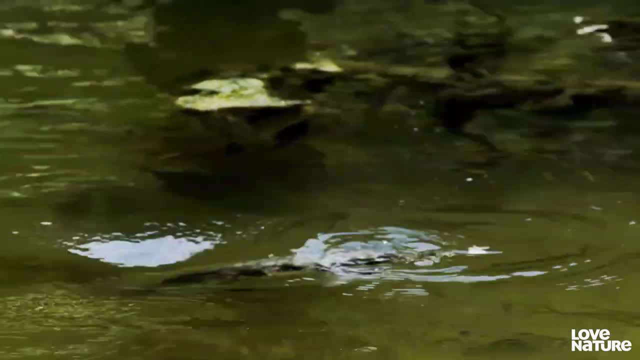 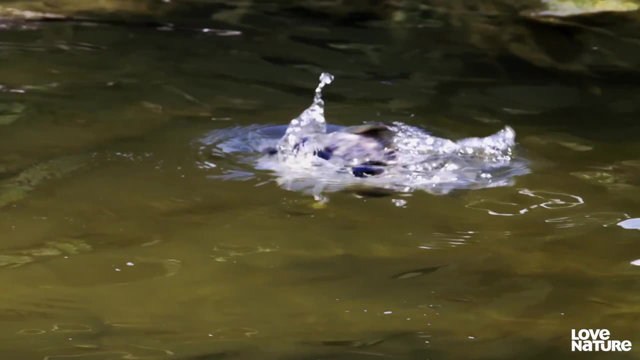 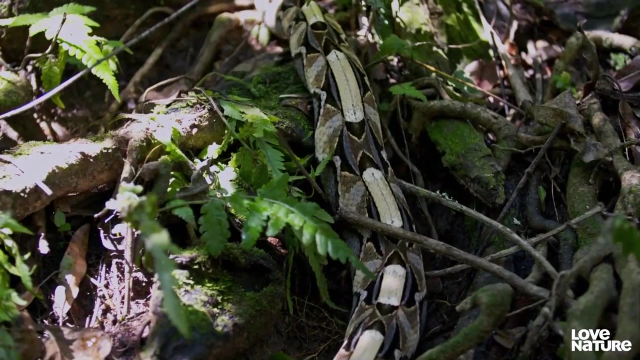 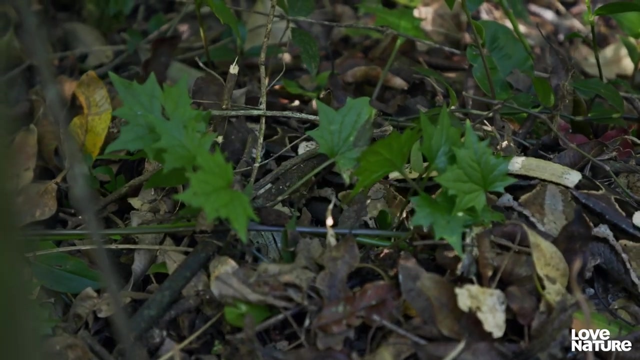 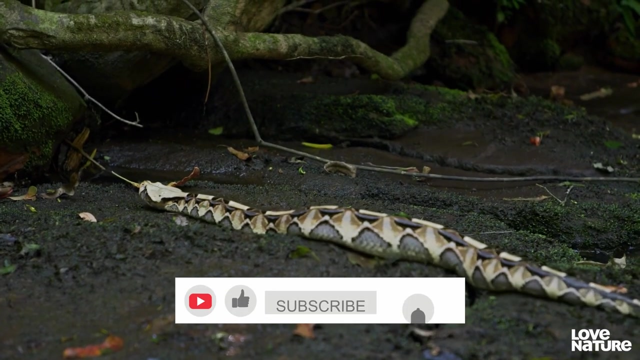 to gauge how much water to fire. Such complex Cognitive behavior makes this miniature sharpshooter one of the smartest fish on the planet. Taking out your dinner at long range is one way to stay safe and save energy, But most predators need to get up close and personal. 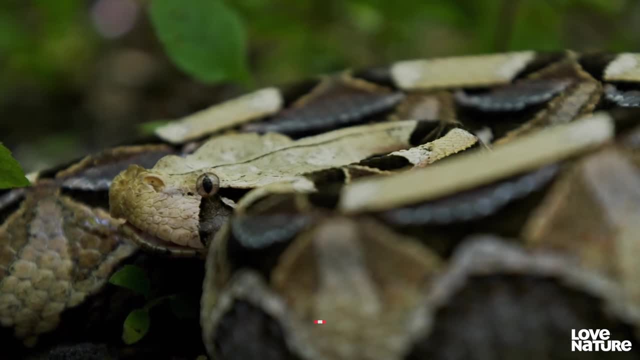 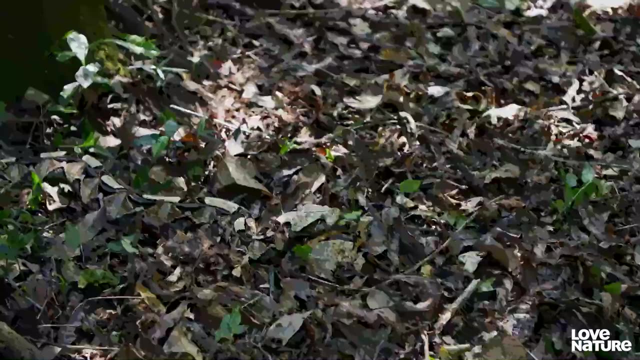 This bruiser is a Gaboon Viper Rippling with muscles. it weighs up to 25 pounds. Its geometric markings mimic fallen leaves- The perfect disguise for an ambush hunter. The Gaboon Viper installs itself near a prey trail. 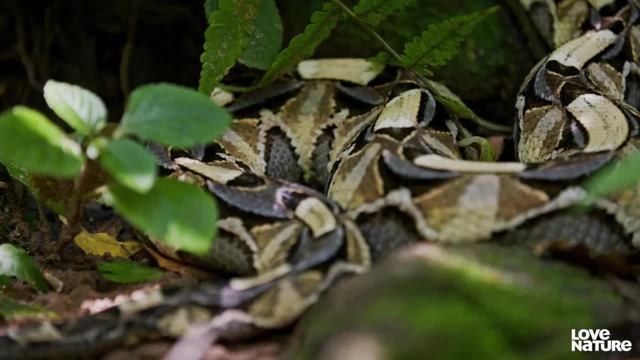 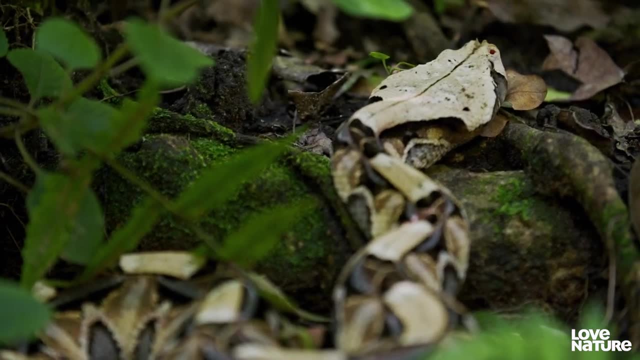 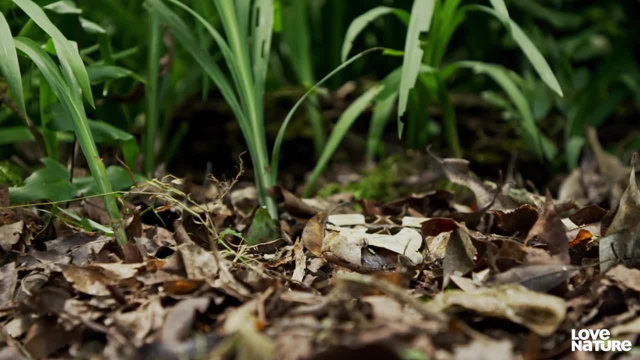 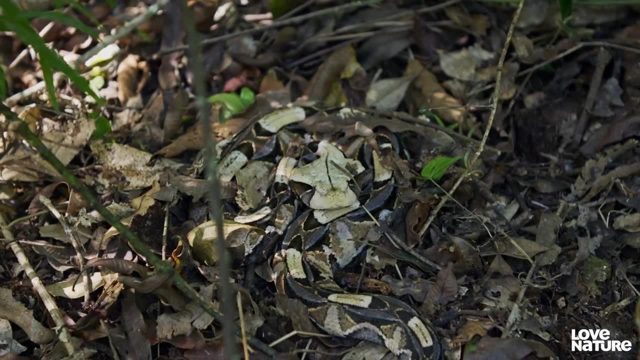 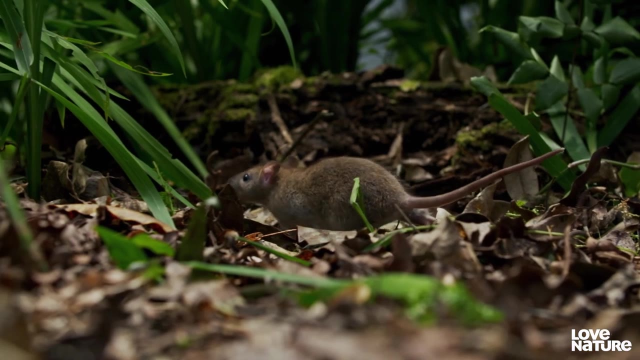 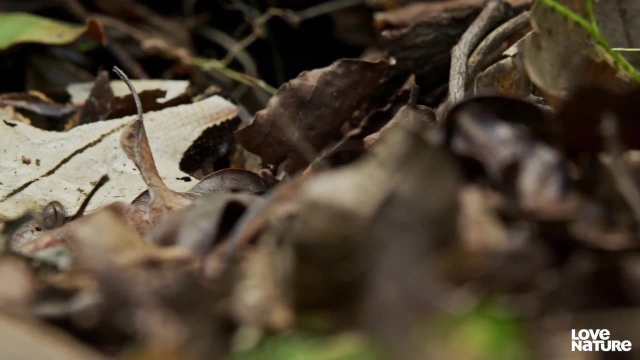 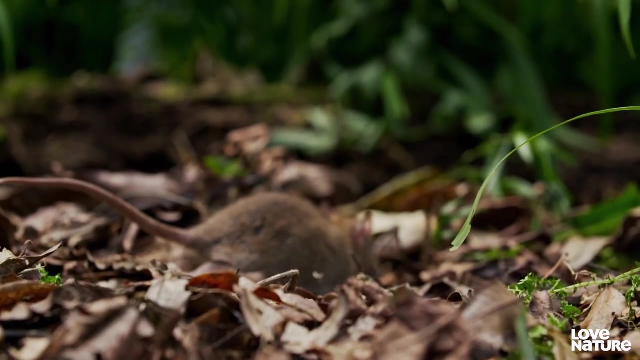 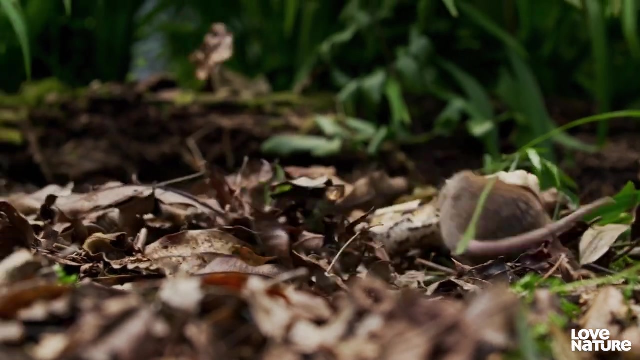 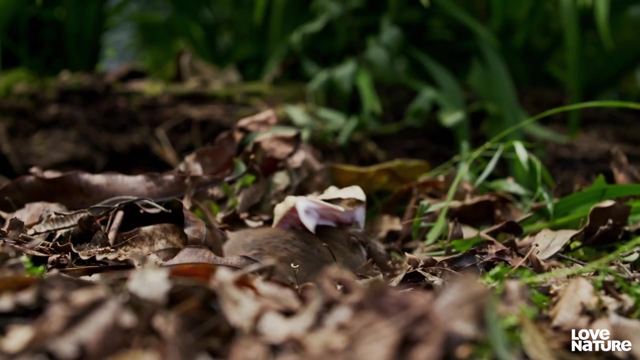 It is a very active predator. It is a very active predator. It is a very active predator. It's armed with thousands of vibration sensors allowing the Viper to tell the difference between approaching danger and approaching dinner. Its two-inch-long fangs- the longest in the snake world. 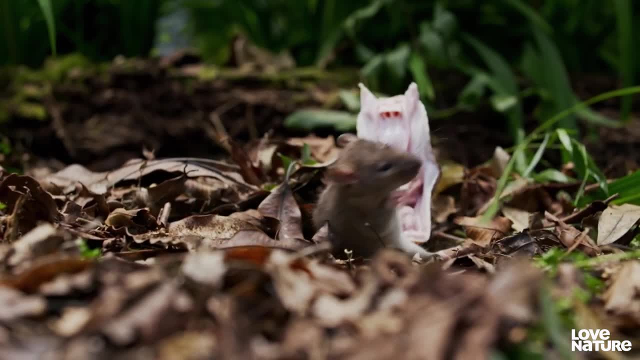 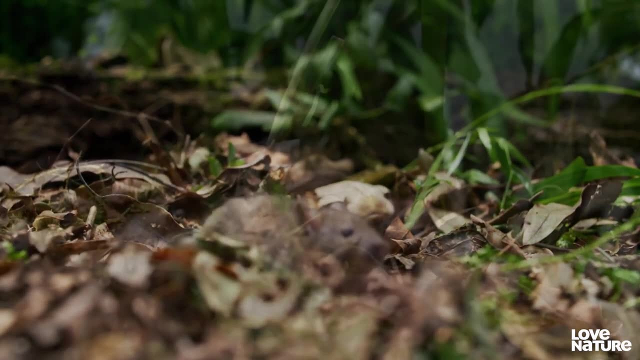 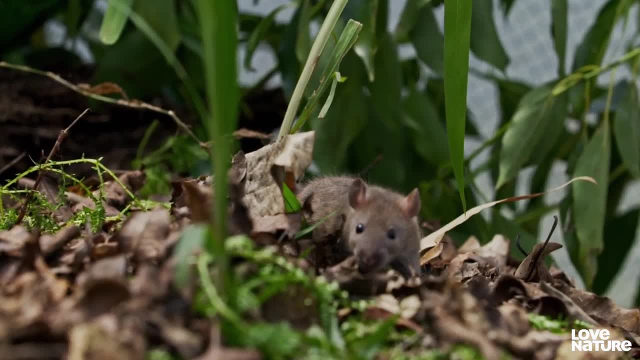 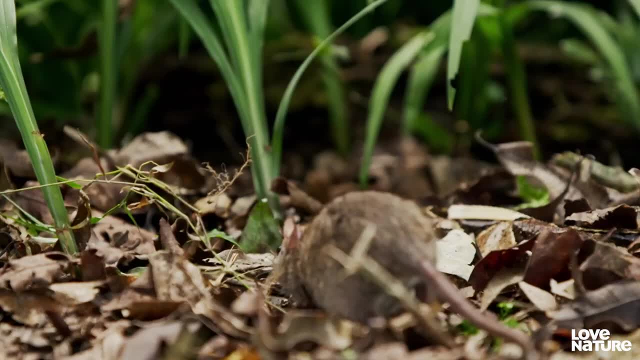 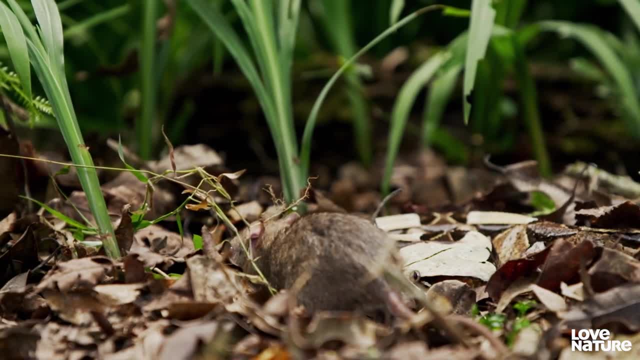 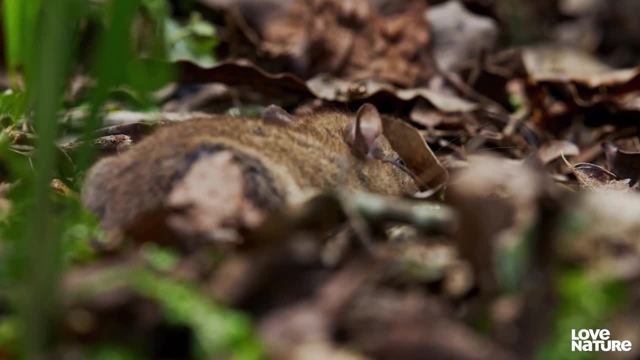 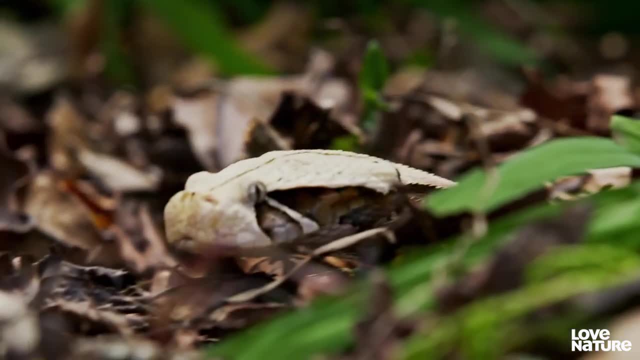 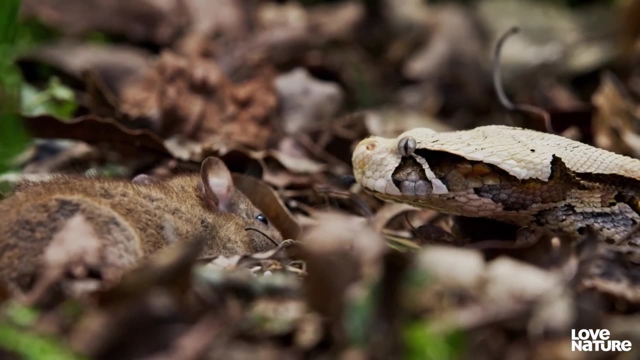 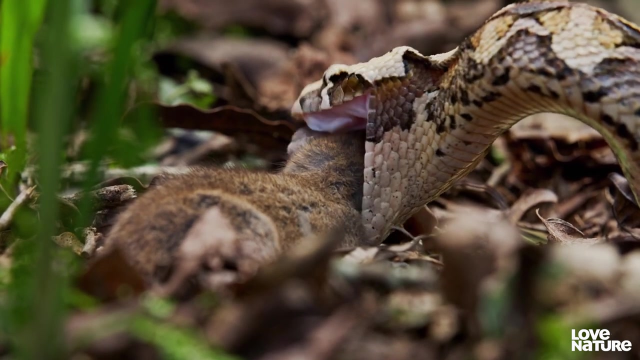 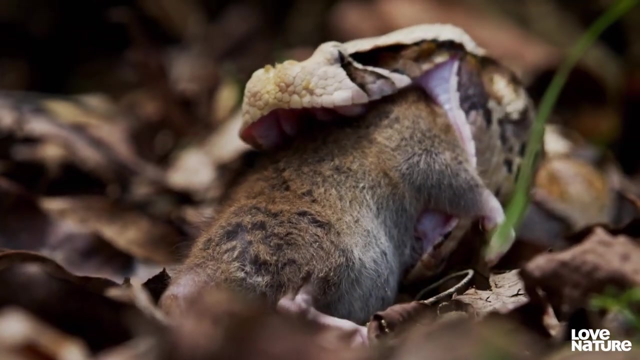 when you can wait and follow the smell of your own venom. Once its prey is unconscious, the snake enjoys its meal in peace. A highly elastic ligament connects its lower jaw to the skull, allowing it to ingest animals wider than its own head. 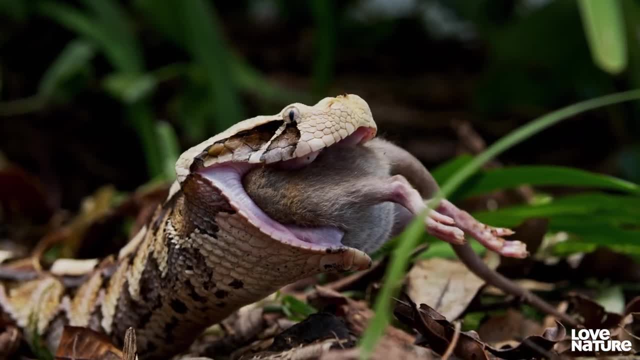 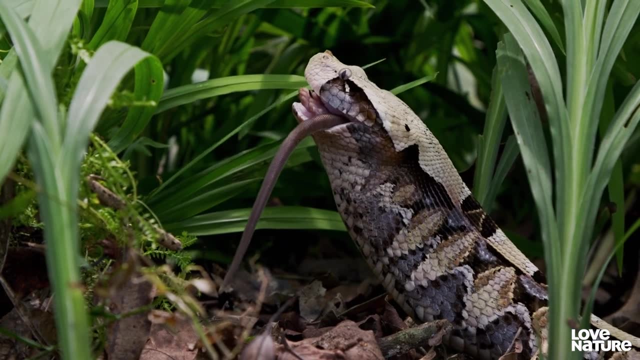 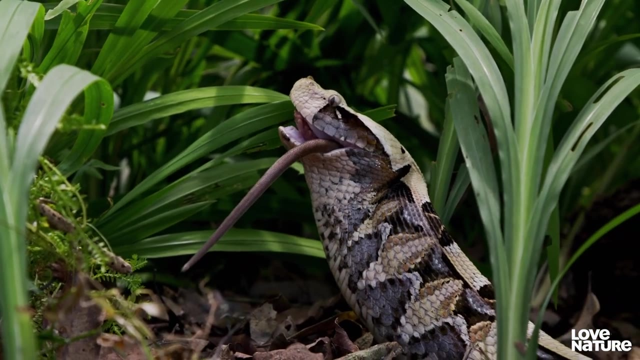 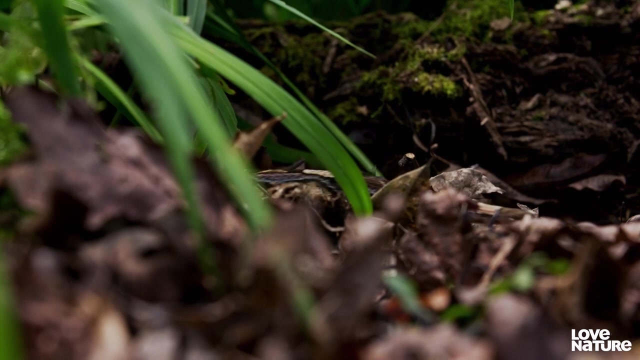 Its huge fangs help claw the rat down its throat. But these blowout meals are only possible because of the venom's final trick. It's still working, breaking down the rat's body, helping to pre-digest the viper's meal. Animal venoms are biological. 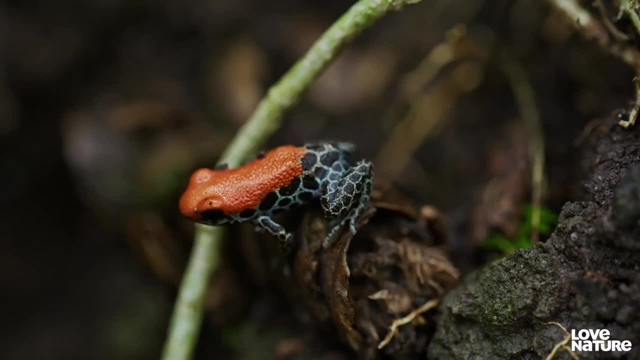 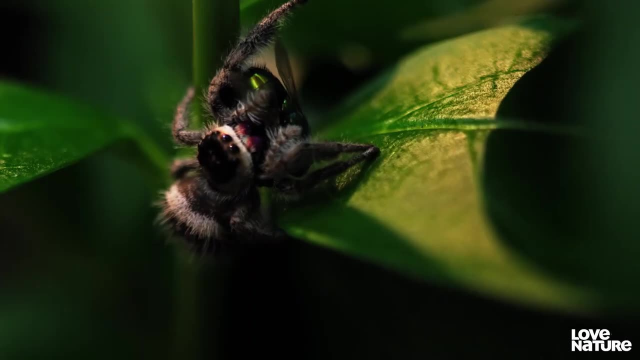 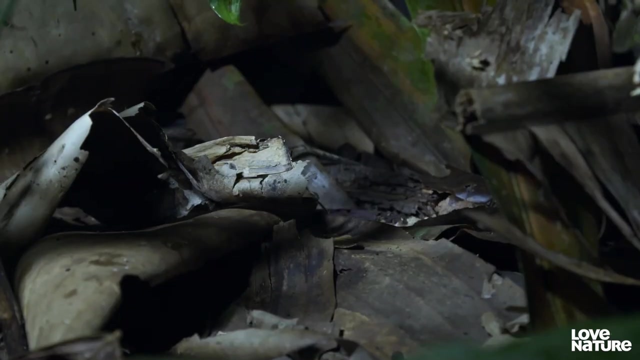 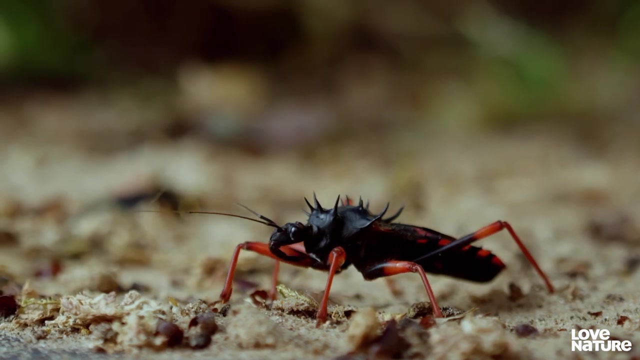 They're substances that were originally designed with different purposes, such as enzymes and hormones, But as their toxic effects on prey evolved, they became an efficient way for predators to dispatch and consume their next meal. This creature's venom does all the hard work when it comes to digestion.